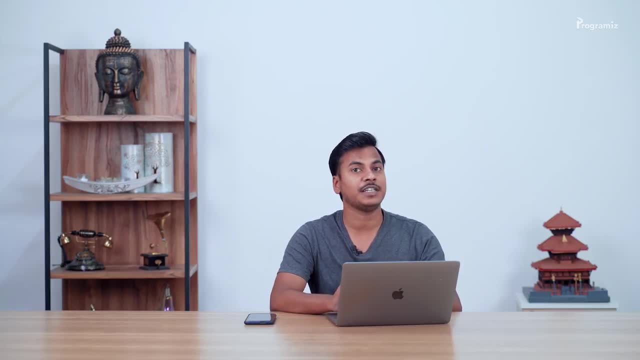 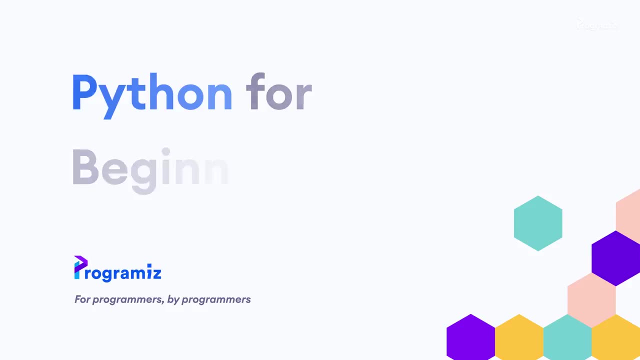 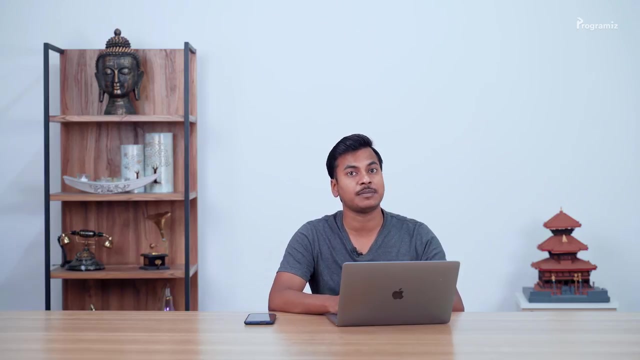 what they are. In this video, we will look into functions in detail and learn how to create them and why they are used. So let's get started In programming. a function is a group of related statements that performs a specific task. They help us divide a large program into smaller chunks so that it's easier to understand. 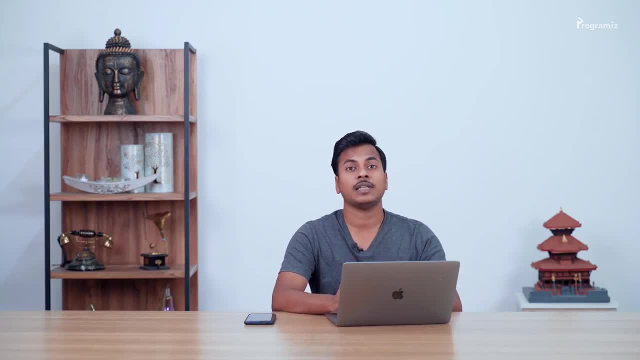 and change. Suppose you need to create a program that draws circles and rectangles of different colors based on user input. Instead of creating one big chunk of statements to create this program, we can create three functions to solve this. First, create a circle function. 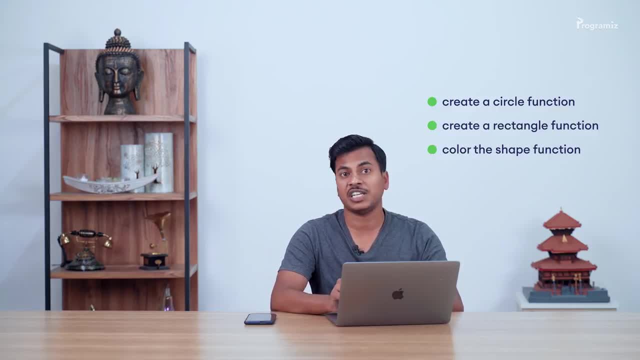 Then a rectangle function And then the color, the shape function. This helps us to divide complexity and we can focus on only a small part of the problem at one time. Now let's see how we can create a function in Python. To create a function, we use the. 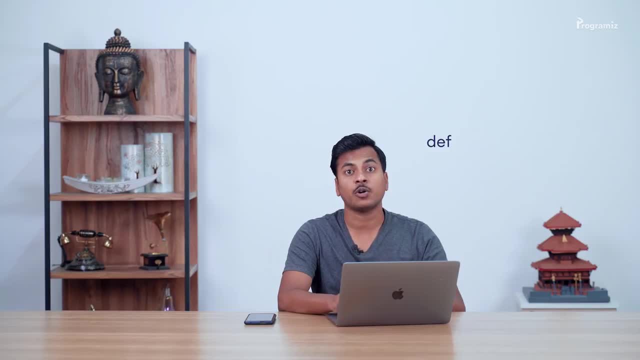 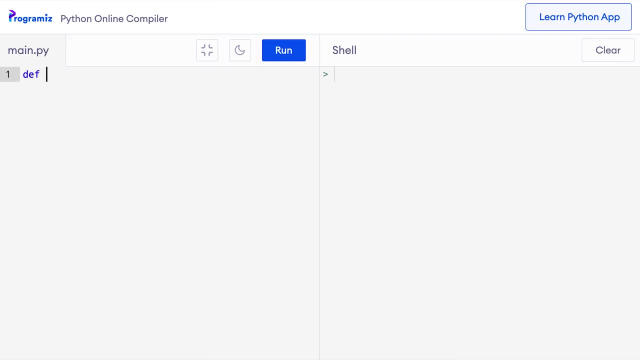 def keyword, which stands for the function definition, followed by the function name, Then I'll use the empty parenthesis followed by a colon. So I'll say def greet- empty parenthesis and colon. Here we have defined a function named greet. However, this code will give us an error because 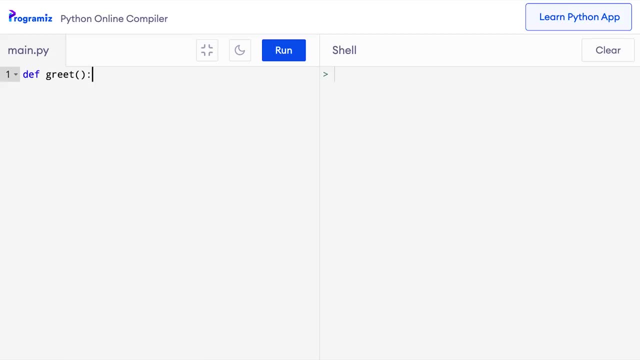 the function body is missing. Let's fix that. For now I'll only add two print statements as its body, So I'll say print hello and then let me add another print statement: print. how do you do? Remember we need to use indentation to specify that this is the body of the function We 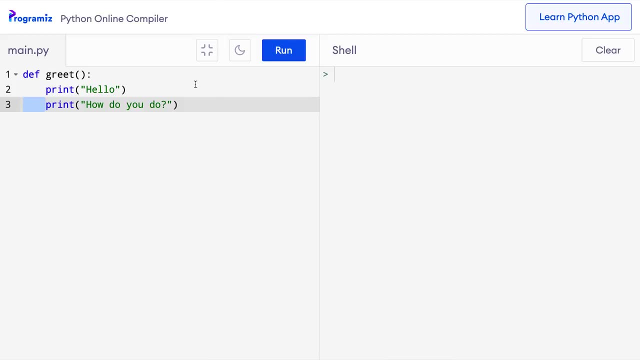 have successfully created a function named greet. Now let me run this code And we don't really see anything. This is because defining a function won't do anything in itself. To bring the function into action, we need to call it. Our function name is greet, with empty parenthesis, So to call it I will just use greet with empty. 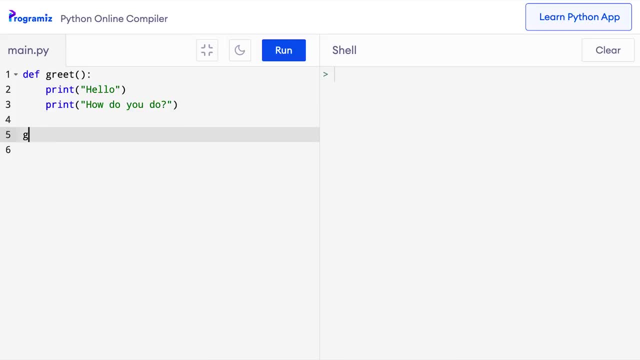 parenthesis. So here I'll say greet, And now, when I press run, then you can see that hello, hello and how do you do? are printed. Here's how this code works. When we call the function, the control of the program jumps. 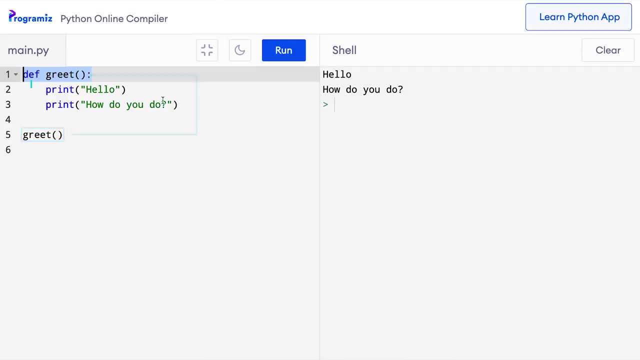 to the function header. Then the statements inside the function are executed. When this task is completed, the control of the program goes back to the function call and the next statement after the function call is executed. One thing with functions is that once we define a function, we can call it any number of times. 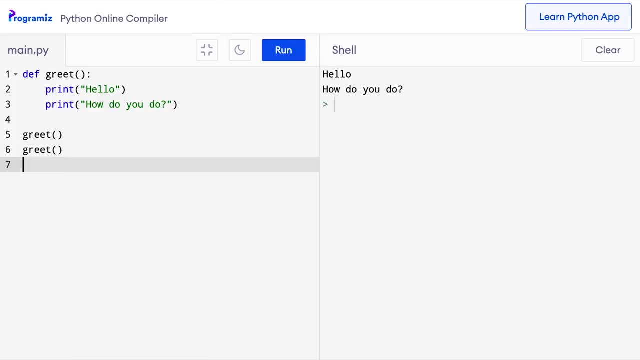 For example, we can call a greet function three times. So here I'll say greet and one more greet, And now, if I press run, as you can see, the function has run three times. That's why these two statements were executed: one, two and three times. 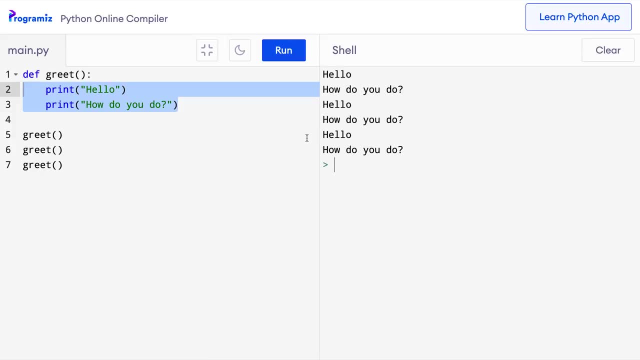 So if we need to perform a task again and again, we can wrap the codes inside a function and use the function any number of times. We just need to call the function again and again. One thing to remember when we create a function is that we need to define a function first. 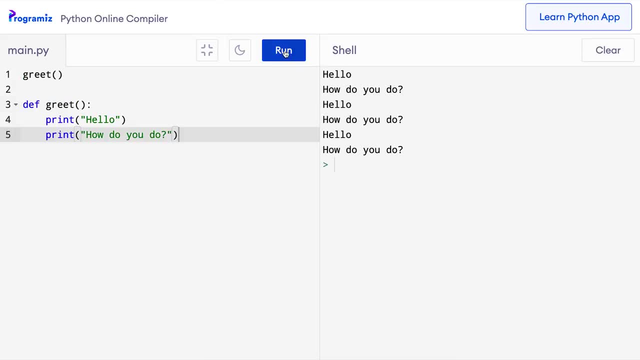 before we can call it. This code, for instance, will not work. Let me run this code to show you Here. when the greet function is called, Python doesn't know that this function exists because it's defined after the function call, So always. 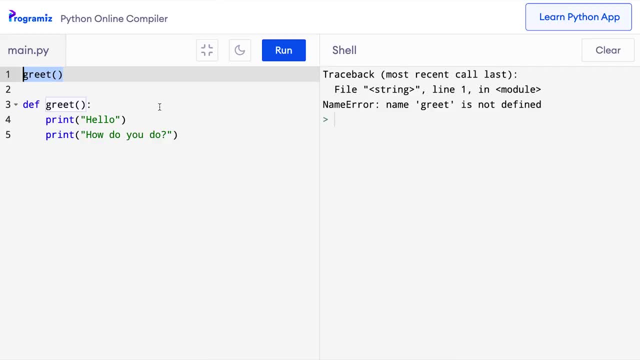 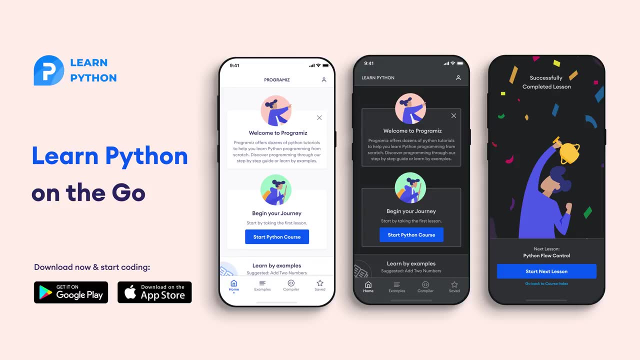 remember to define a function before you use it. Before moving to the next section of the video, I'd like to mention that the programmers team has created an app that allows you to create a function and use it for any task. You can use this app to learn Python from your phone. The app contains bit-sized lessons that are 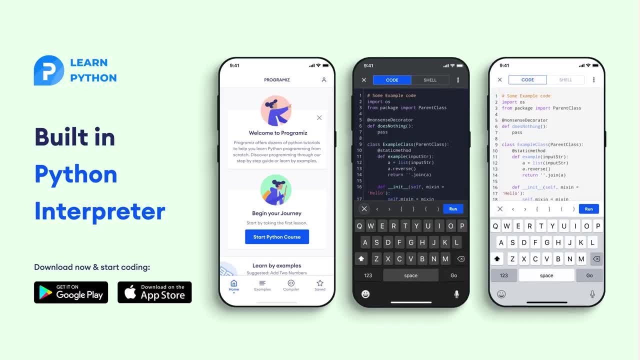 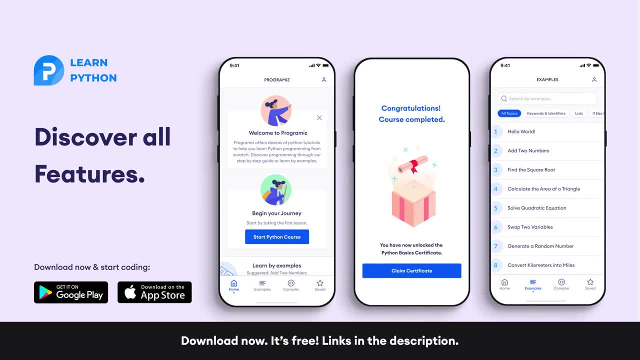 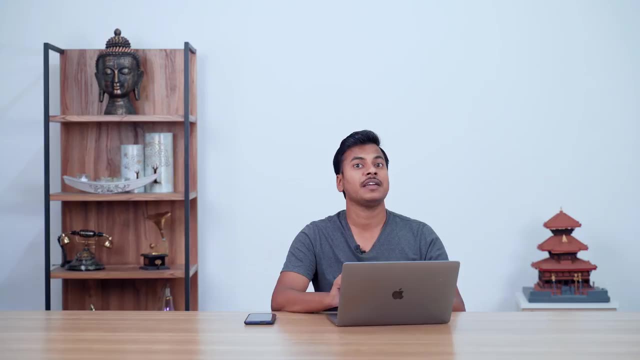 easy to understand, a built-in interpreter so that you can run Python on your phone, quizzes and many more features. The app is available on both iOS and Android. The links are in the video description below. Now let's talk about Python arguments and how our greet function. from the previous example, 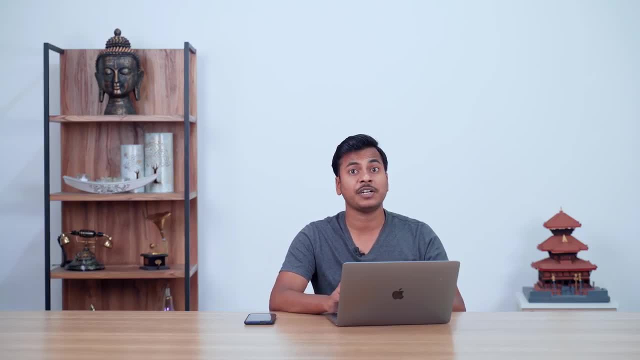 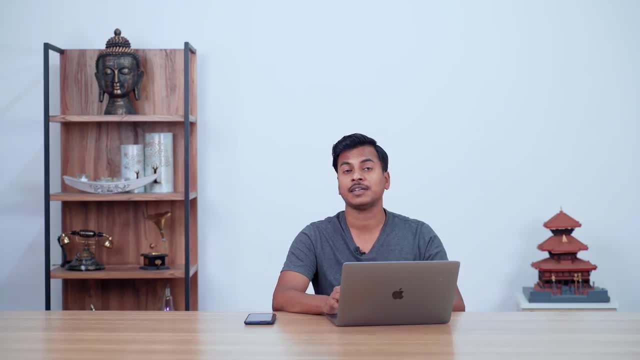 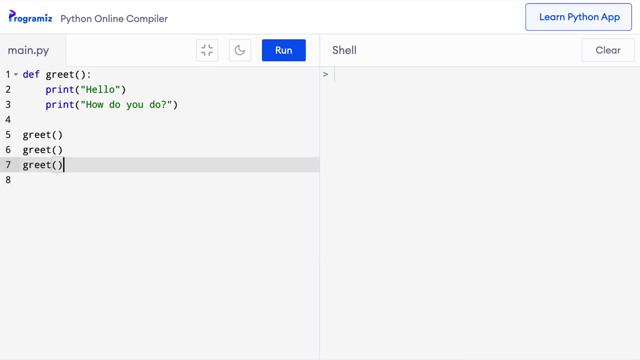 Or we can print something like hello, jack or whatever the person's name is. In such cases, we can pass values to a function. These values that we pass to a function are called arguments, So I'll go back to the code that I started with. I'll remove these two greet functions. 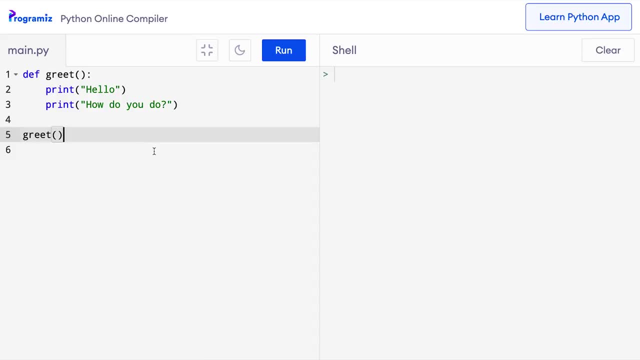 because I want only one, and here inside the greet function I'll pass the jack string like this: This value that we passed during a function call is called an argument. So jack, here is an argument, And in the function definition I'll add a variable in the greet function. 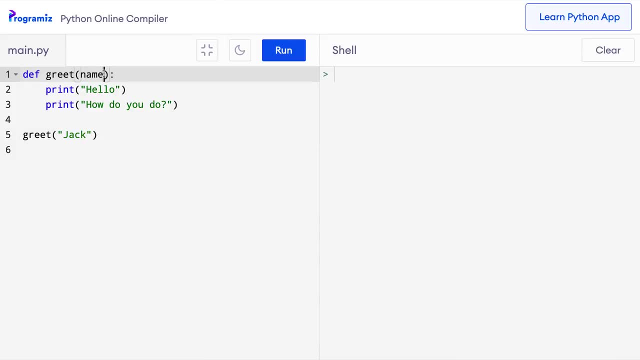 I'll call it name. This name variable accepts whatever value is sent as an argument during the function call. In this case Jack is transferred to the variable name. Now I can use the name parameter inside the function. So now I can say hello comma name and when I press run then I get hello Jack. 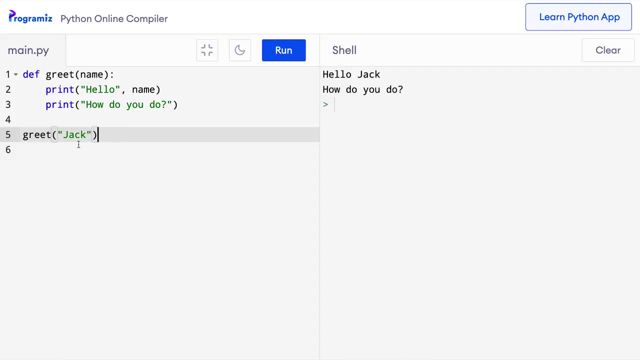 Let's see step by step how this function works. When we call the greet function with the argument Jack, then this is passed to the name variable inside the function definition. Then the statements inside the function are executed. We can use the name parameter inside the body of the function. 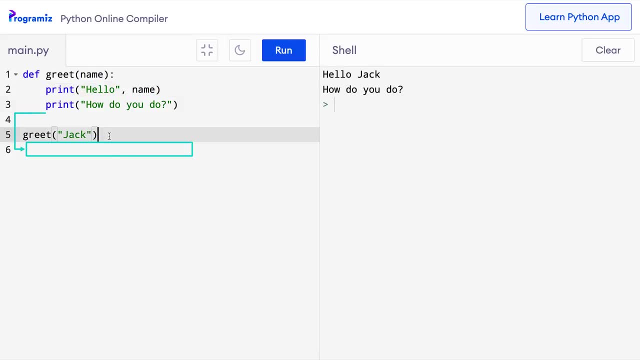 When this task is completed, the control of the program comes back to the place from where the function was called and the next statement is executed. In this case, there's nothing here. It's also possible to pass multiple arguments to a function, as per our needs. 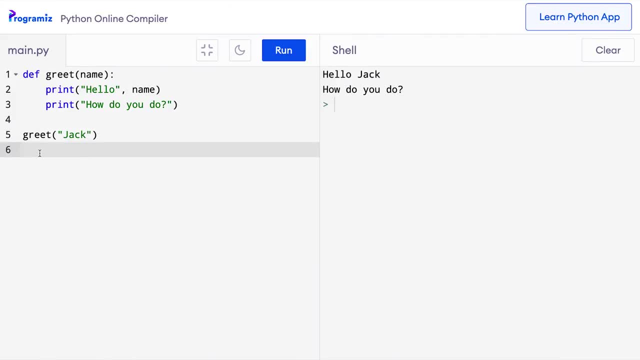 If we need to pass multiple arguments to a function, we can separate them by commas. Let's see this in action by creating a function to add two numbers. So I'll remove the old code and I'll create a new function called add numbers. 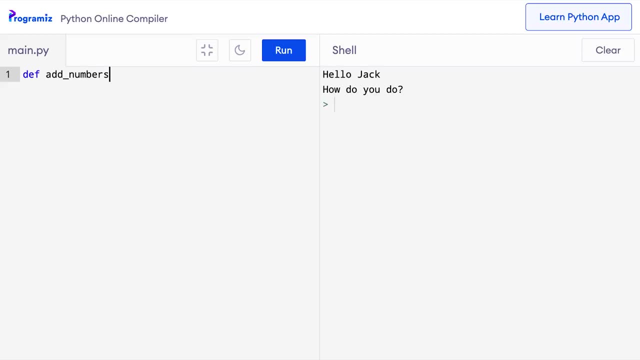 So I'll say def- add underscore numbers. Obviously I'll need two parameters: n1 and n2.. And then inside the function I'll say result equals. And then inside the function I'll say result equals. I'll say result equals n1 plus n2.. 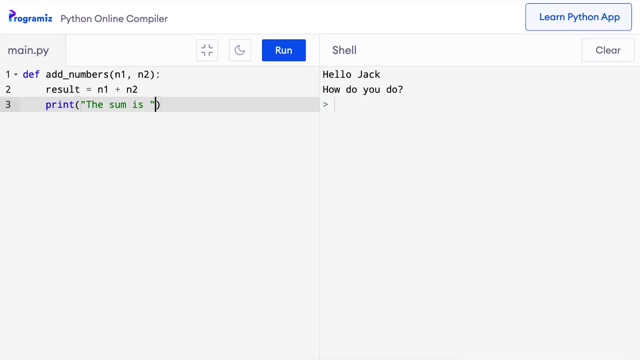 Print the sum is, and here I'll say result. Now, outside the function, I'll say: number one equals 5.4,, number two equals 6.7, and then I can call add underscore numbers: Number one, comma, number two. In this program we have passed number1 and number2 as arguments to the addNumbers function. 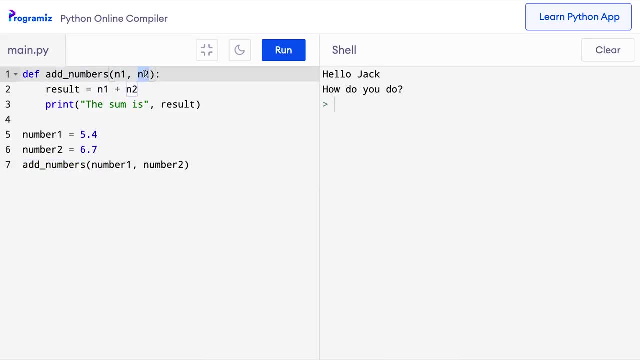 These arguments will be accepted as n1 and n2 once they are passed to the addNumbers function. So inside the function n1 will be 5.4 and n2 will be 6.7.. Then we have added the numbers and printed them inside the function itself. 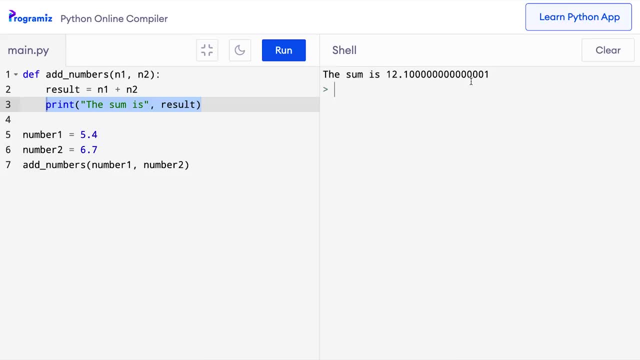 Let's run this code and see the output. As you can see, I now have the sum of those two numbers In our program to add two numbers. we are finding the sum of numbers and printing it. It's working fine. However, it's better just to find the sum inside the function and print the result somewhere. 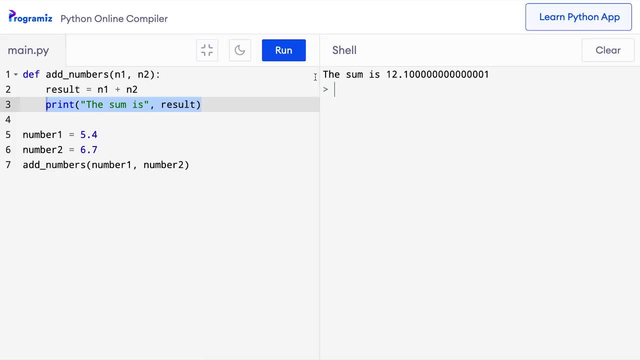 else. We can achieve that by using the return statement Inside the function. I'll remove this print statement and I'll say: return, return, return, return, return, return. When we return a value, it comes back to the function and we can assign this return. 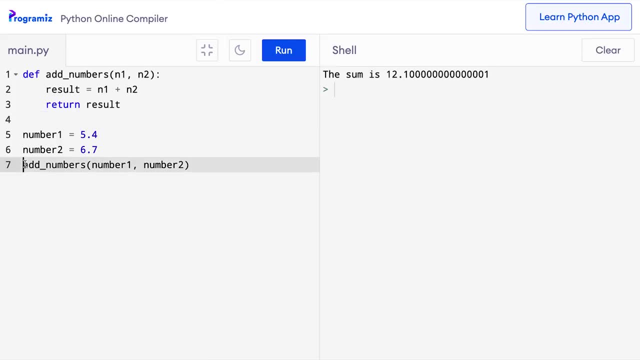 value to a variable like this. So here I can say: result equals addNumbers And I can print the result as print the sum is, and then I can say result. Let's see step by step how this program works. We call the addNumbers function with two arguments. 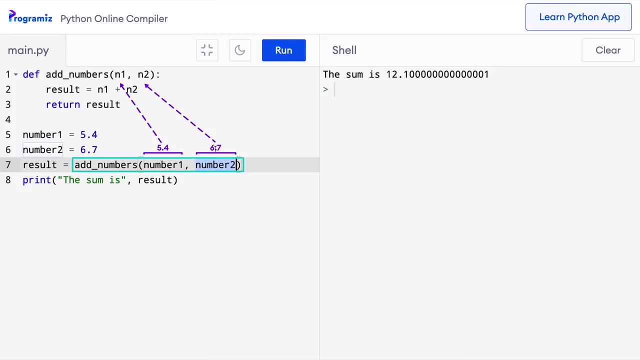 Number 1 and number 2, which are accepted by the function definition as n1 and n2.. The sum of n1 and n2 is calculated and the result is returned to the function call. This return value is assigned to the result variable. 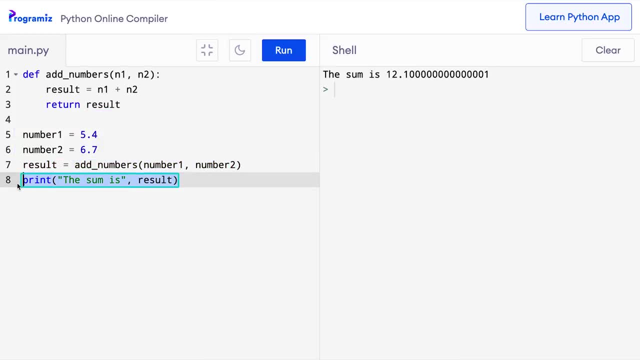 And in the next line we just print the result variable outside the addNumbers function. Whenever a return statement is encountered inside a function, the control of the program goes back to the place from where it's created. Let's see an example of this. 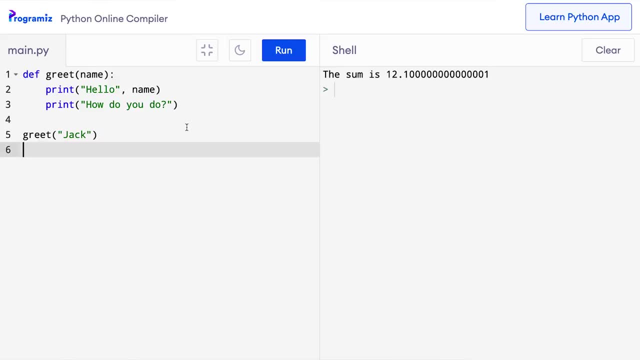 Let's get back to our greet function that we wrote before. I'm pasting it here. When I press run, then we get: hello, Jack, and how do we do here Now? let me modify this program a little bit. I'll add a return statement after this line and let's see what happens. 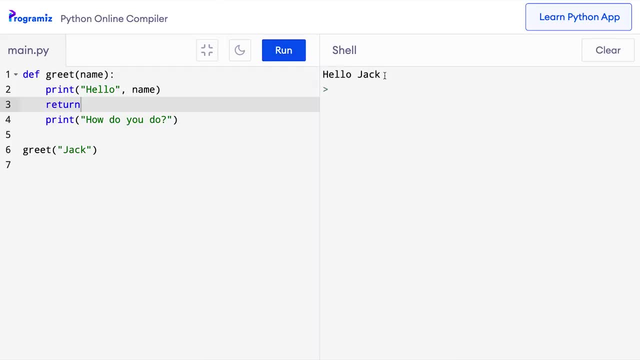 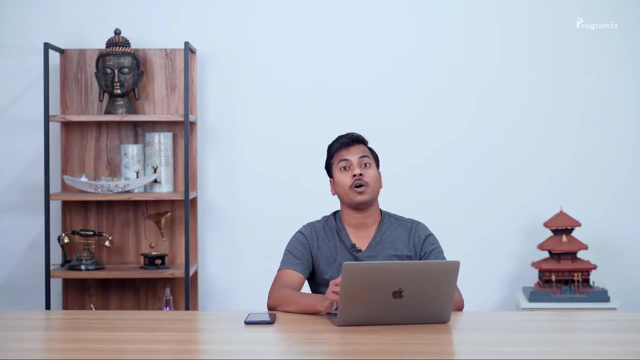 Now, when I press run, then you can see that only hello Jack is printed. This is because when the return statement is encountered Immediately, the function terminates and control of the program goes back to the place from where the function is called. At this point we have covered all the basics to create a function. 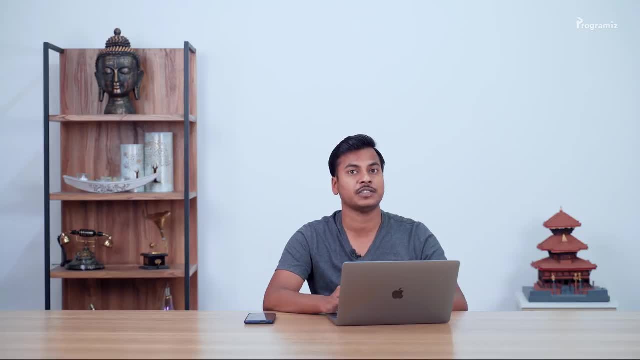 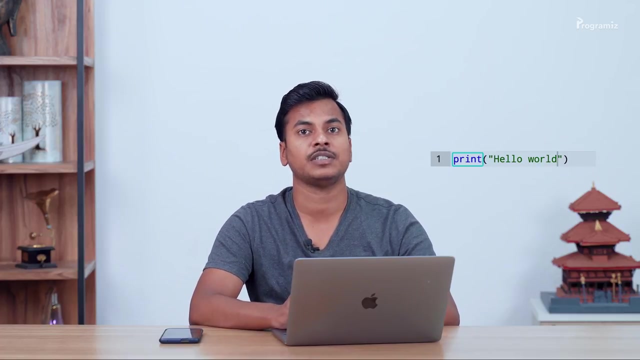 These functions we created ourselves are known as user defined functions. Actually, we have already used functions numerous times in all of our videos. Remember print? It is also a function. The function definition of this print statement is defined somewhere inside the Python programming language. 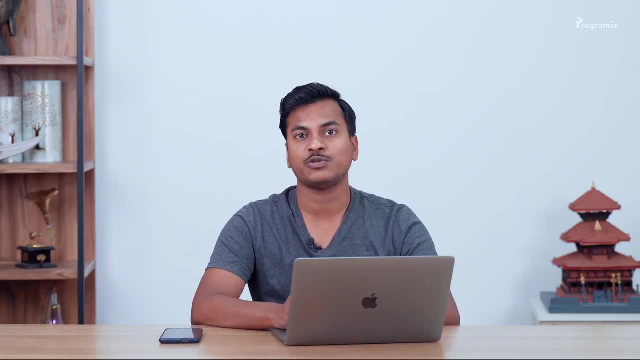 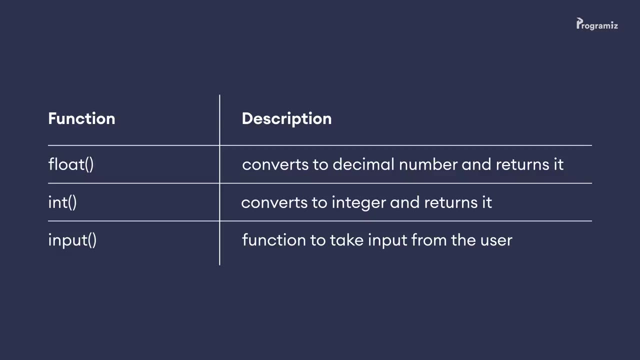 That's why we can just call the function and it just works. These functions defined inside of Python are called built-in functions. We have also used other built-in functions, like float, int input and so on, in our videos. There are numerous built-in functions available in Python that make our life a whole lot easier. 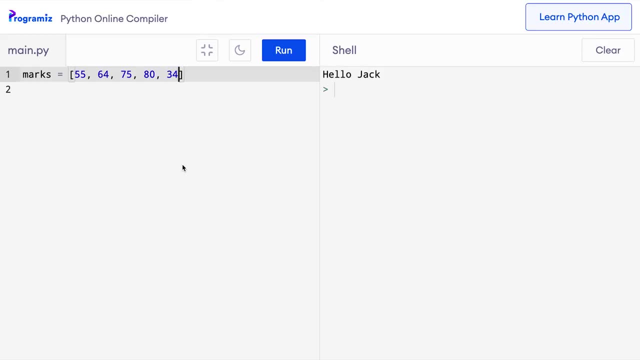 For example, suppose we have a list like this: If we need to find the length of this list, we can use the len function. So here I can say length equals len marks And I can print the length of the list, as print length is comma length. 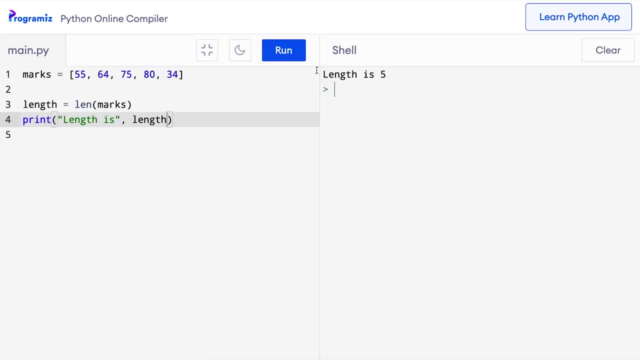 Let's run this code and see the output. When I press run then, as you can see, it says length is 5, which is the length or the number of items in this marks list. If we instead needed to find the sum of the items of the list, 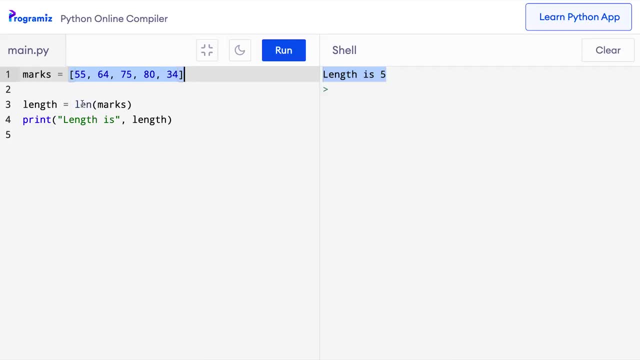 We don't need to manually write the code ourselves. We can use the sum function that's available in Python. So here I can say: marks underscore sum equals sum of marks, And then I can print the sum as print. the total marks you got is. and then I can say: 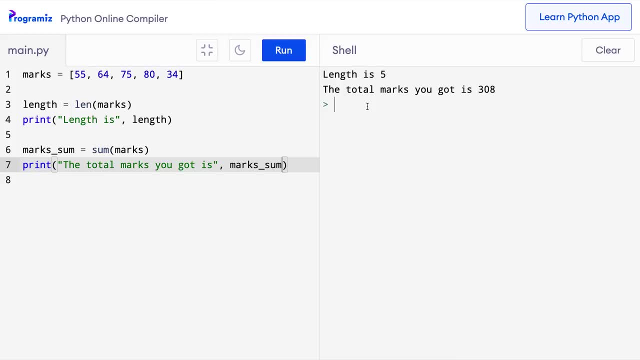 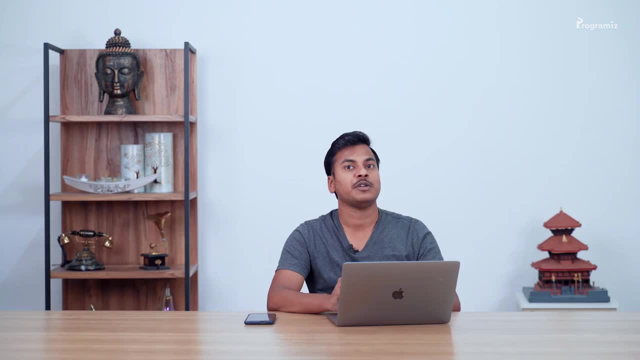 marks underscore sum. Now when I press run, then it says the length is 5. And the total marks you got is 308, which is the sum of these marks. If you are interested, you can find all the built in functions available in Python in: 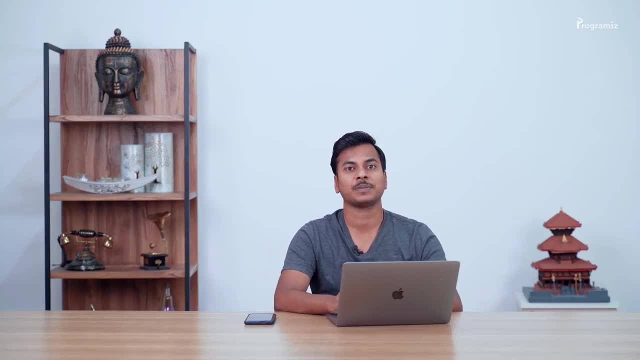 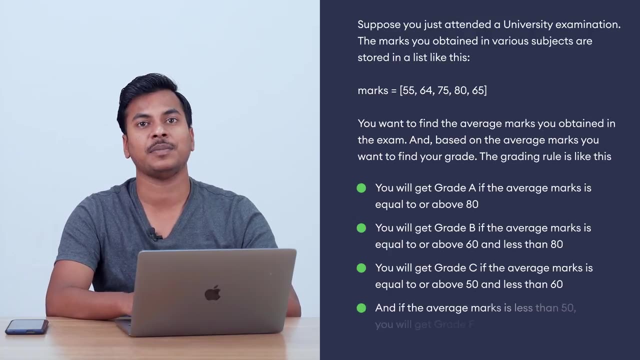 the programmerscom website. The link will be in the description below. Let's put all the things we have learnt in this video in action. Suppose you have just attended a university examination. The marks you obtained in various subjects are stored in a list like this: 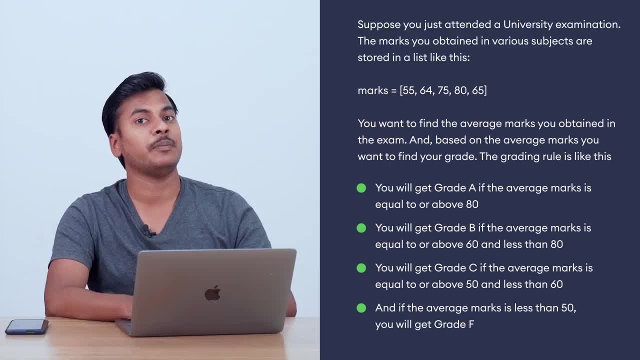 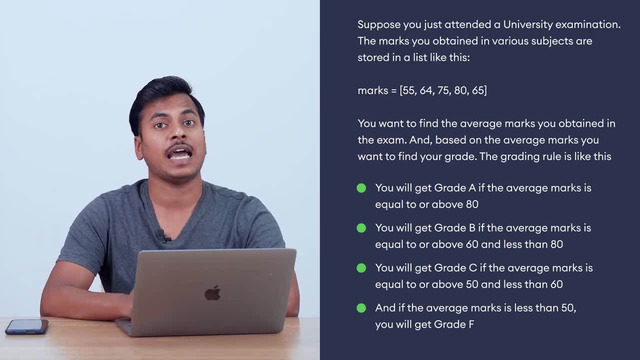 You want to find the average marks you obtained in the exam And, based on the average marks, you want to find your grade. The grading rule is like this: You will get grade A if the average marks is equal to or above 80.. 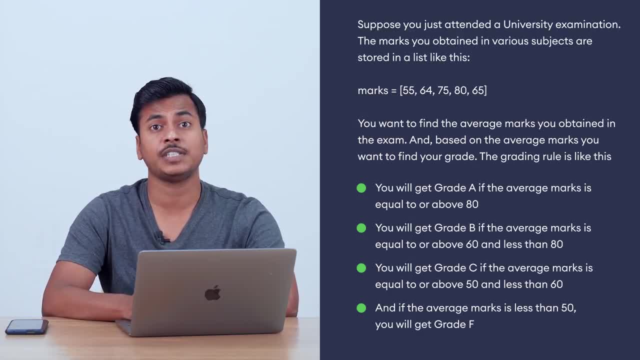 You will get grade B if the average marks is equal to or above 60 and less than 80.. You will get grade C if the average marks is equal to or above 50 and less than 60. And if the average marks is less than 50, you will get grade F. 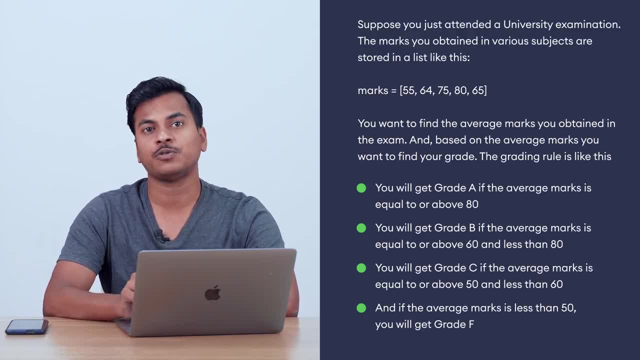 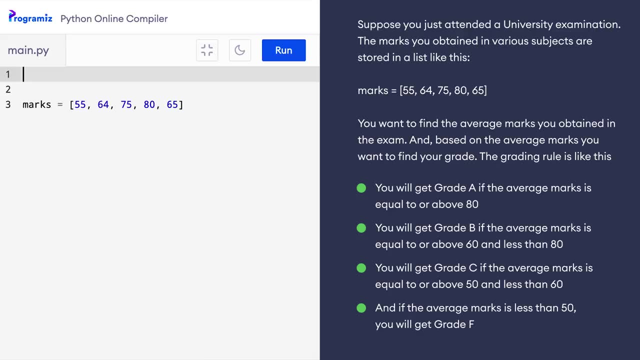 To solve this problem, we will create two functions: 1. One to find the average marks and another to compute the grade. So let's get started. I will start with the function definition, But before that let me add a little comment. 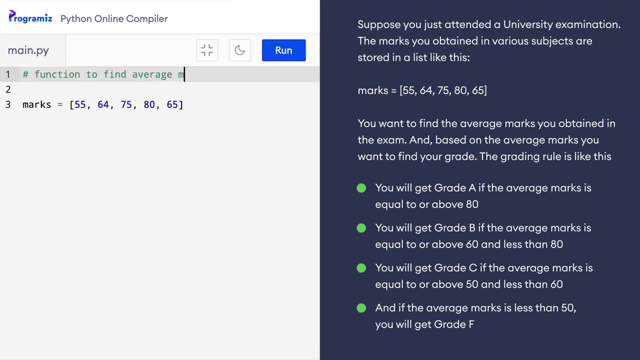 I will say function to find average marks. Let me define my function as def- find average marks. Now the argument to this will be a list of marks and inside I will say: sum of marks equals sum marks. I also need to find the number of subjects or the number of marks I have. 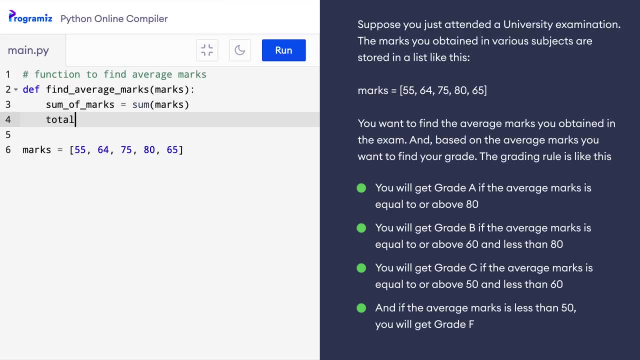 So I will say: total underscore subjects equals the length of this marks list, And then now I can calculate the average, as average underscore marks equals sum of marks divided by total subjects. Let me return this average marks variable And now, outside the function, I can say: 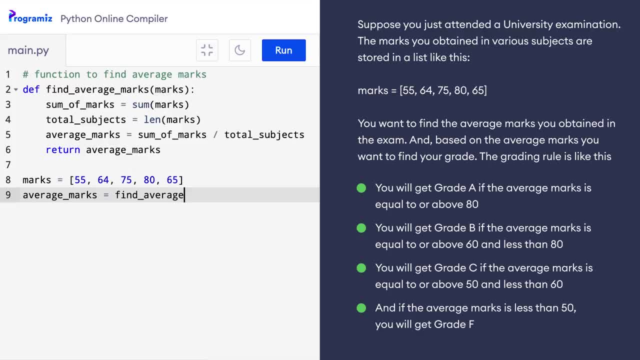 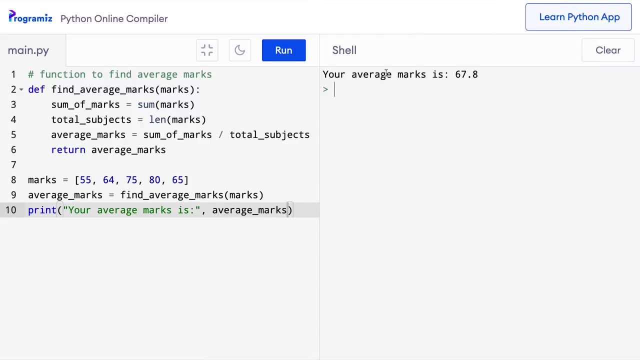 Average marks equals: find average marks. I will pass in the marks list And here I will say: print your average marks is and I will say average underscore marks. When I press the run button I can see that my average marks is 67.8, which is the average. 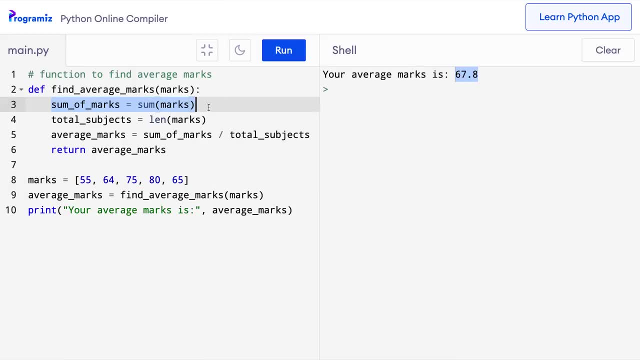 of these five numbers, Which is calculated as sum of these numbers divided by the total number of subjects, which is 5 in this case. Now we need to create another function to calculate the grade based on the average marks. Let's do that now. 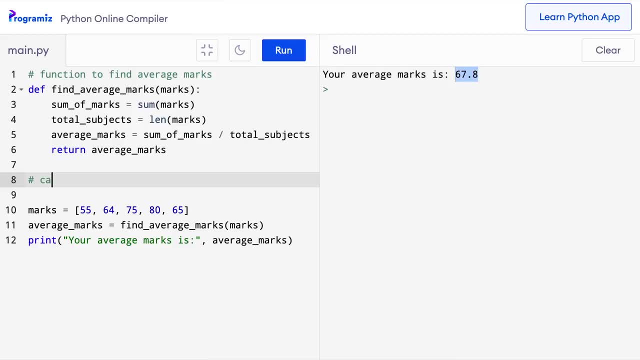 I'll create another function, But before that let me add a little comment. I'll say: calculate the grade and return it, And then I'll say: def: compute underscore grade. Now the parameter or the argument to this will be the average marks. 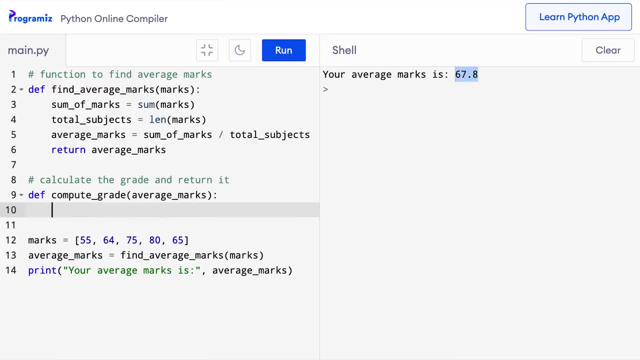 So I'll say average marks And inside I'll say If Average Marks Greater than equals 80. Then grade is A- Elif average marks greater equals 60.. Then the grade is B- Elif average marks greater than equals 50. 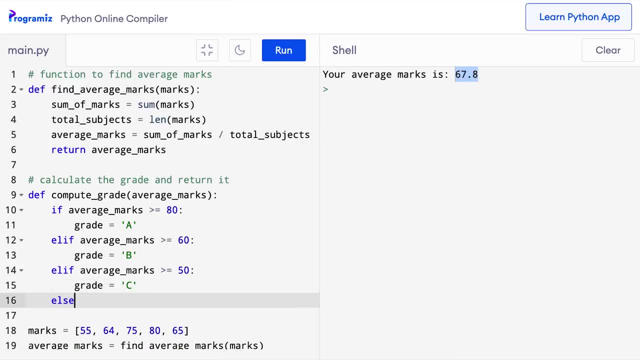 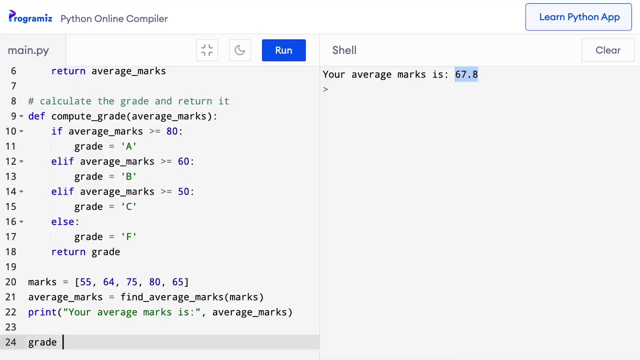 In this case the grade is C And the else clause, I'll say Grade equals F And outside the if block, I'll say return grade. Now I can use this computeGrade function as grade equals, compute underscore, grade, average marks. 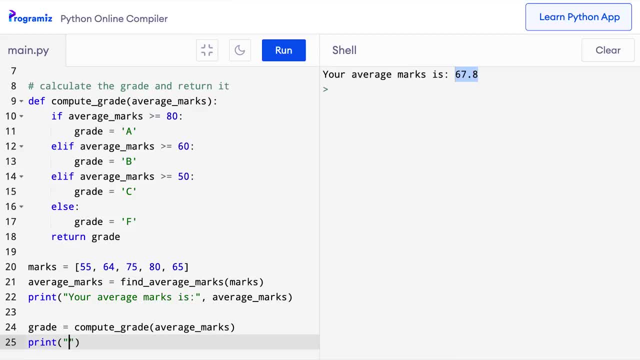 Now let me print this grade as your grade is and the grade variable. Now, when I press run, The grade is And the grade variable, And when I press run, I can see that my average marks is 67.8 and my grade is B, Which is not the best result. 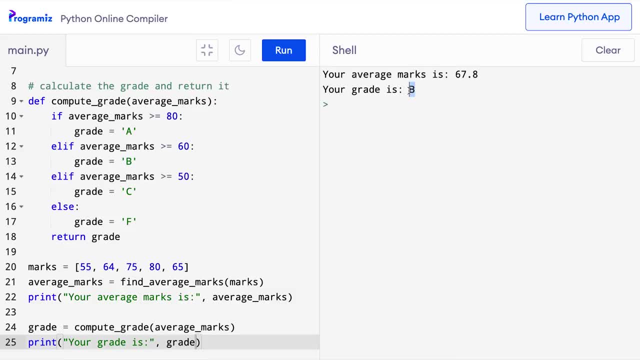 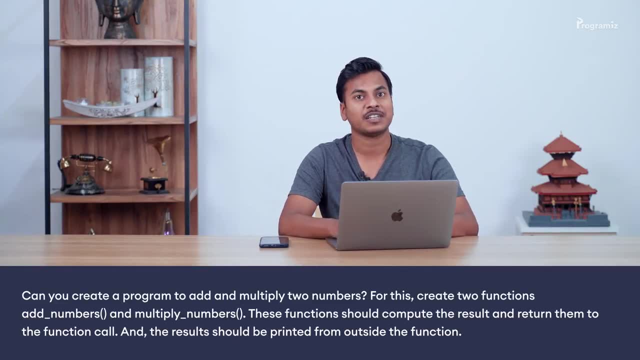 but at least I now know what my grade is. Before we end this video, here's a programming task for you. Can you create a program to add and multiply two numbers? For this, create two functions: add underscore numbers and multiply underscore numbers. 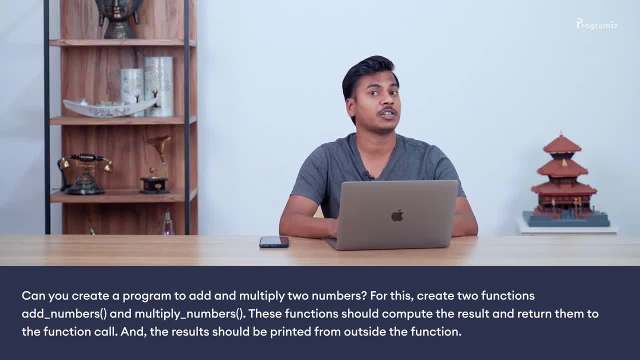 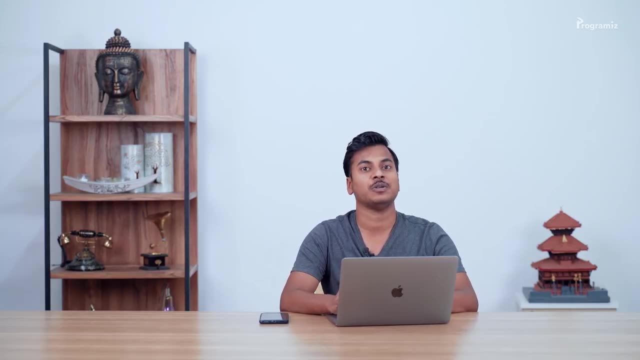 These functions should compute the result and return them to the function call, and the results should be printed from A to Z. You'll find the answer to this question in our Github repository. Also visit our website, programmerscom, for more tutorials and examples. The links will be in the description below. 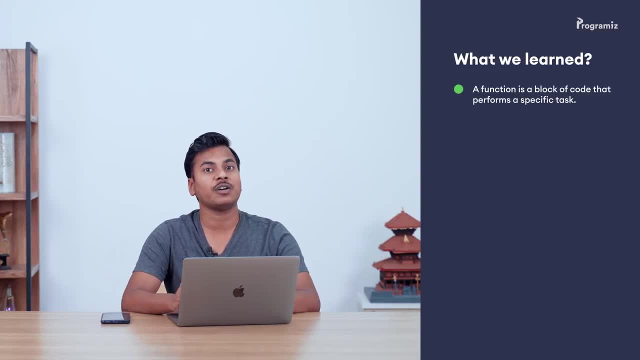 Now let's recap what we learned. A function is a block of code that performs a specific task. We use the def keyword to define a function. To bring the function into action, we need to call the function. We can call the same function as many times as we want, as per our needs.